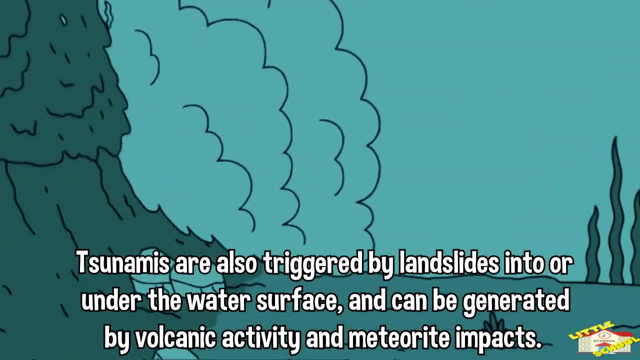 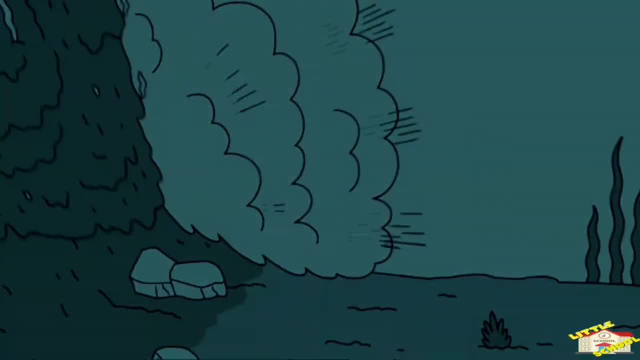 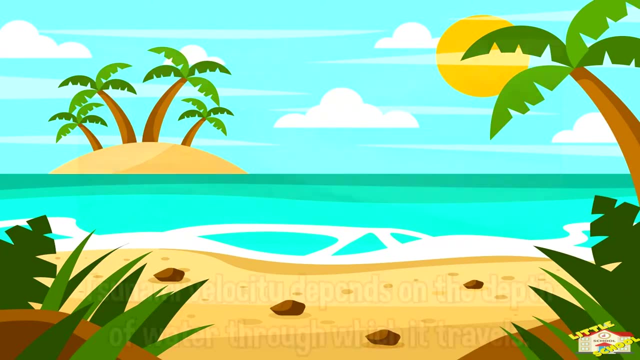 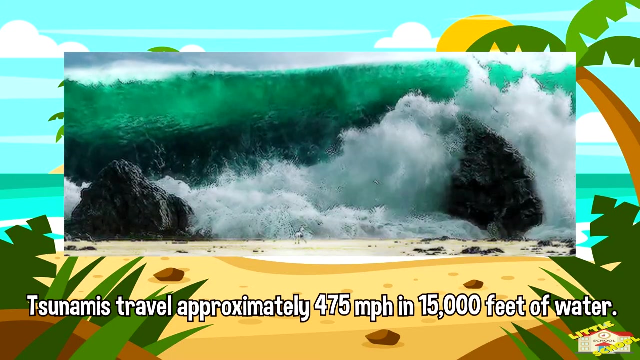 Tsunamis are also triggered by landslides into or under the water surface and can be generated by volcanic activity and meteorite impacts. How fast do tsunamis travel? Tsunami velocity depends on the depth of water through which Tsunamis travel: approximately 475 miles per hour in 15,000 feet of water. 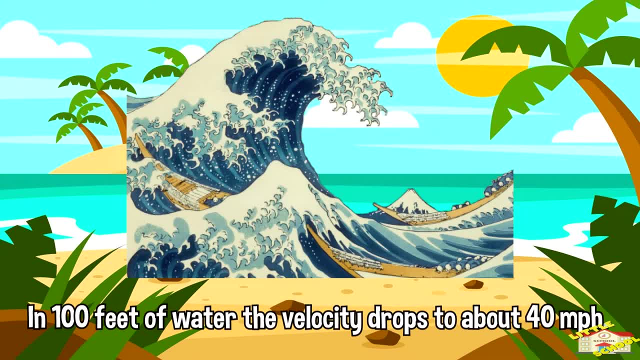 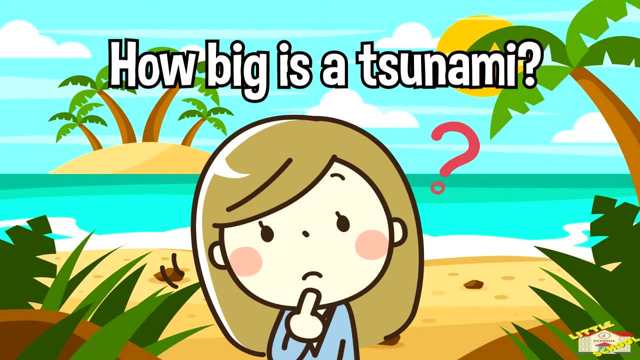 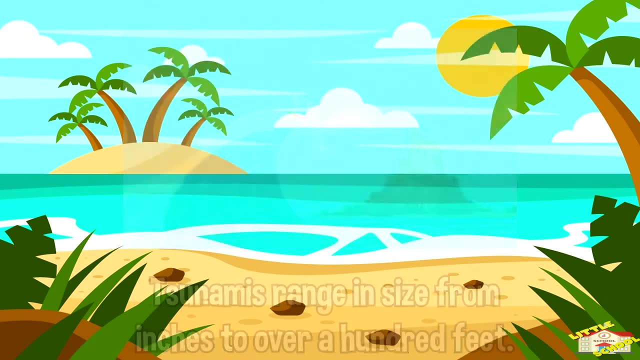 In 100 feet of water, the velocity drops to about 40 miles per hour. How big is a tsunami? Tsunamis range in size from inches to over 100 feet. In shallow water, the top of a wave moves faster than the bottom of a wave, which is 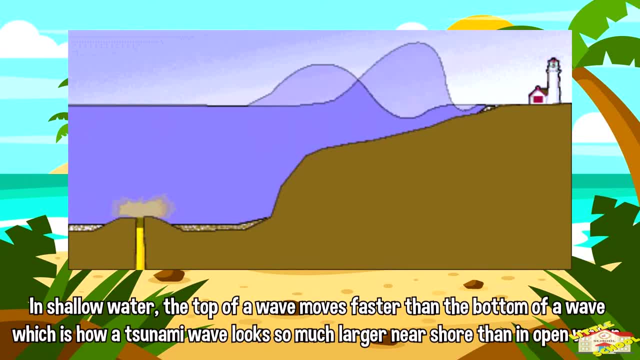 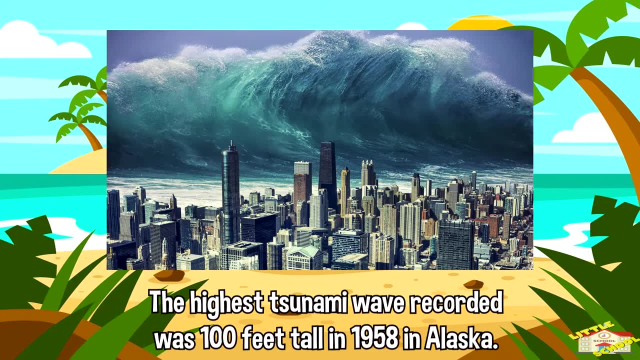 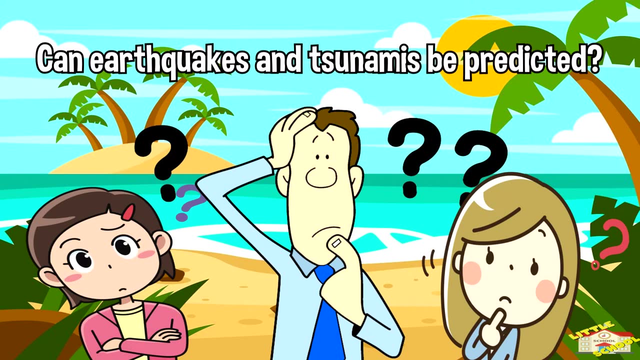 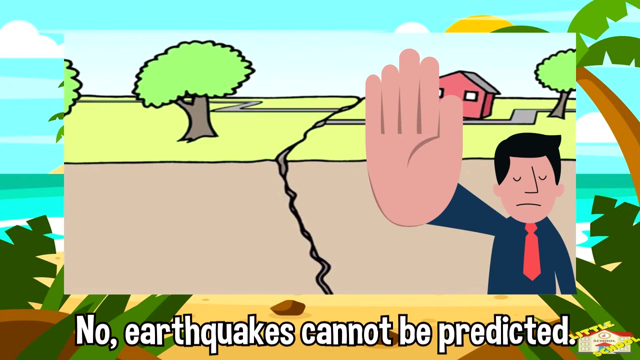 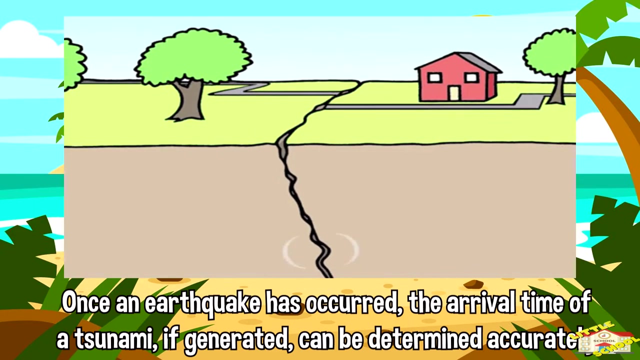 how a tsunami wave looks so much larger near shore than in open water. The highest tsunami wave recorded was 100 feet tall in 1958 in Alaska. Can earthquakes and tsunamis be predicted? No, earthquakes cannot be predicted Once an earthquake has occurred. the arrival time of a tsunami, if generated, can be determined. 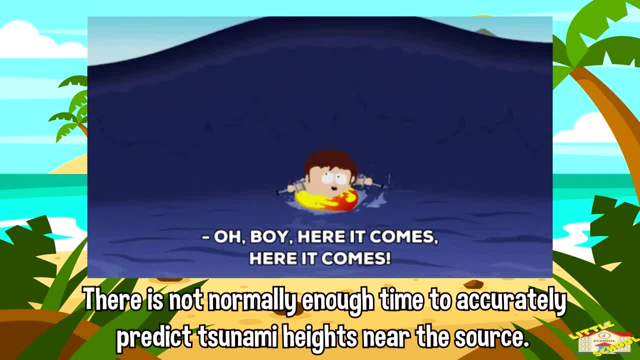 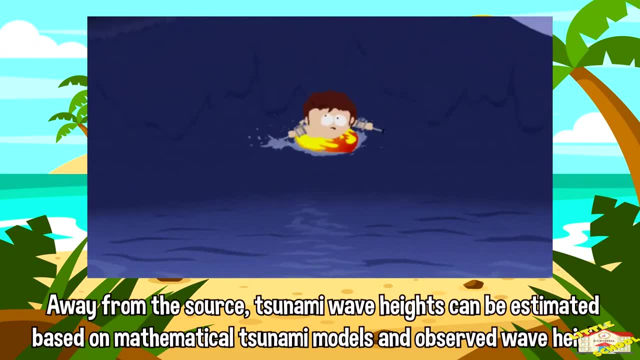 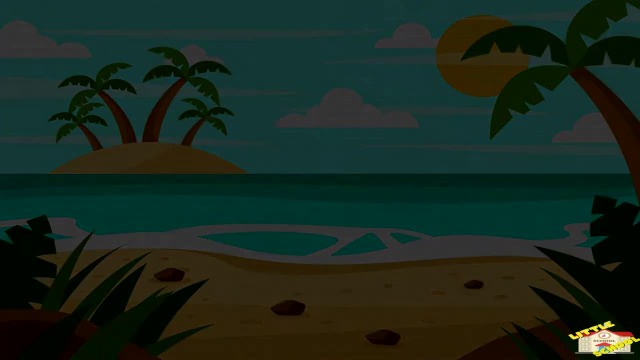 accurately. There is not normally enough time to accurately predict tsunami heights near the source. Away from the source, tsunami wave heights can be estimated based on mathematical tsunami models and observed wave heights. How big is a tsunami? Up to about 3.3 million times the size of a tsunami. 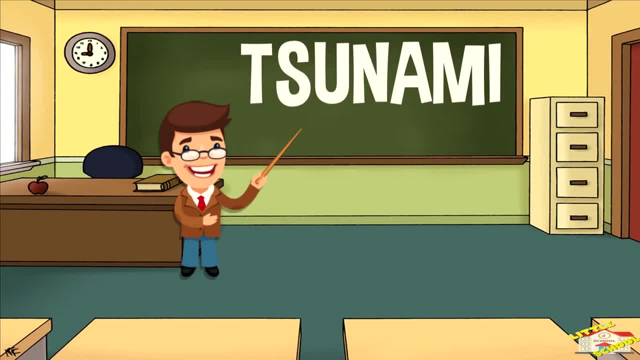 The highest tsunami velocity is the longest tsunami wave in our time. The video is up to about 1.5 million times the size of a tsunami. In this video I wrote about how an earthquake could change the life style of a tsunami. I hope you enjoyed learning about tsunamis today. 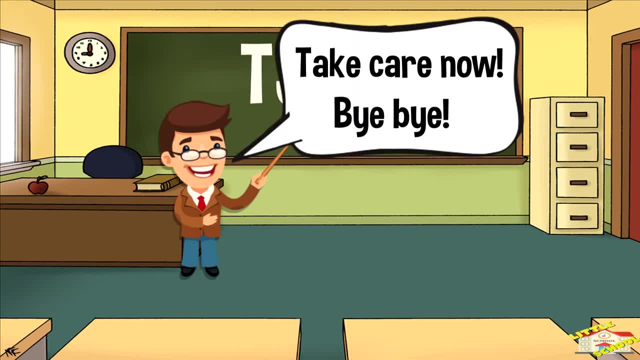 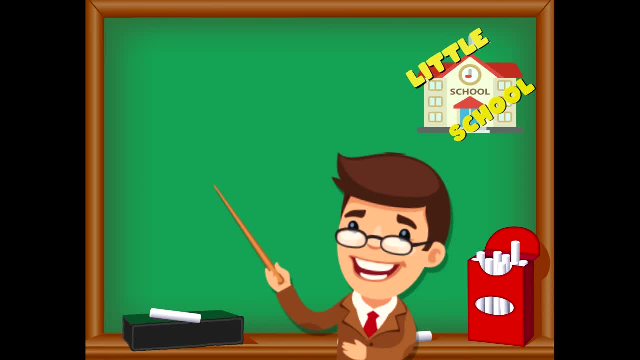 Stay tuned for more. I hope you also have a good day. Thanks for watching. If you enjoyed the video and want to see more videos from us, please click the subscribe button. Also, give us a like. that will help us. We thank you so much and we do hope that you. 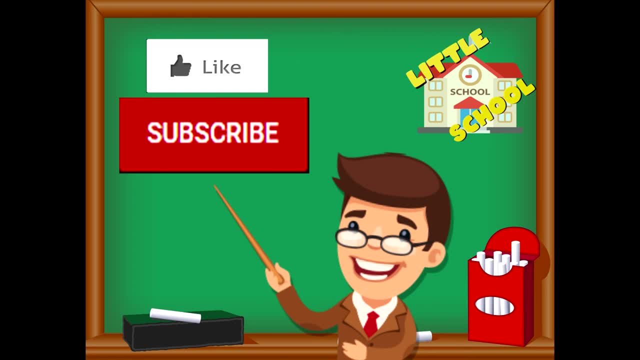 enjoy our videos. See you soon. Thanks for watching.